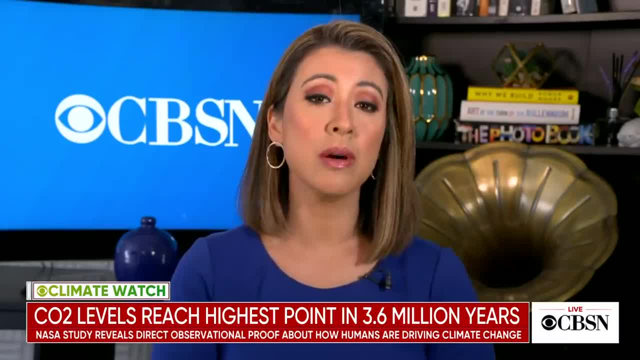 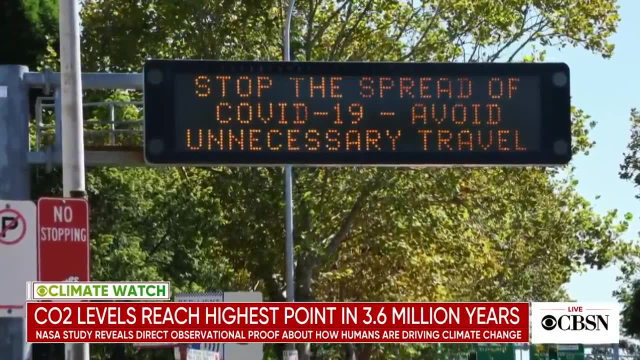 The amount of carbon dioxide pumped into the Earth's atmosphere was lower than scientists originally estimated for 2020.. Researchers say the pandemic helped to keep the numbers down, But this isn't all good news. Scientists also warn that CO2 levels are at their highest point. 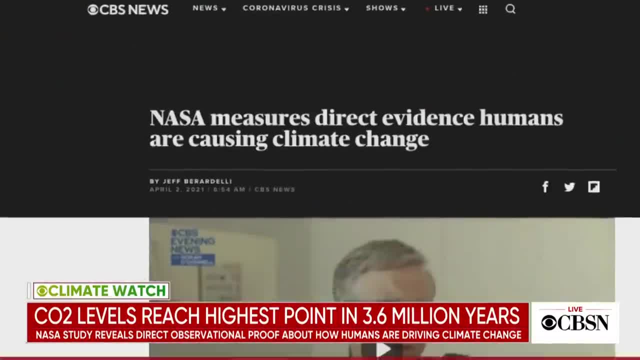 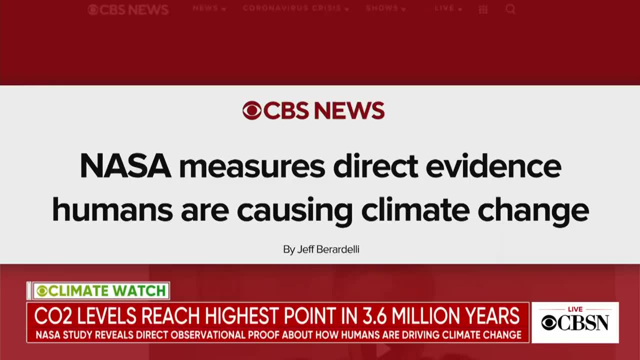 in 3.6 million years. Now, for the first time, NASA is placing scientific blame on people in its new study looking at what drives climate change through direct observations. For more on this study, CBS News meteorologist and climate specialist Jeff Berardelli joins me now. 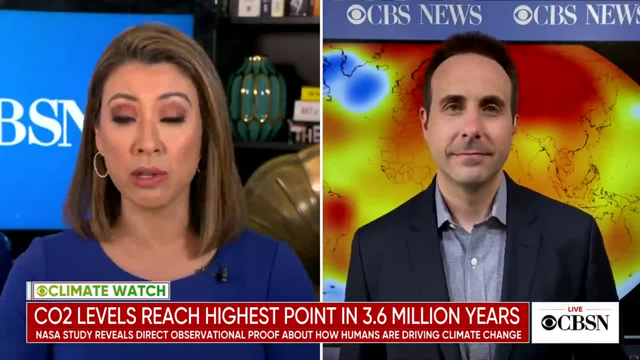 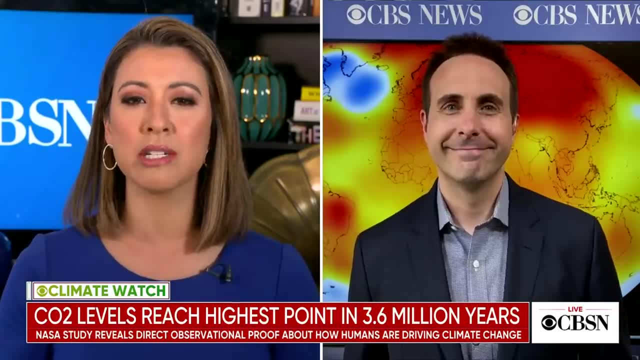 Jeff, help us understand this. Because of the pandemic, CO2 levels were lower than expected. That makes sense, But still they're at their highest point. How do these two seemingly contradictory facts coexist? That's because the atmosphere is kind of like a bank account, So 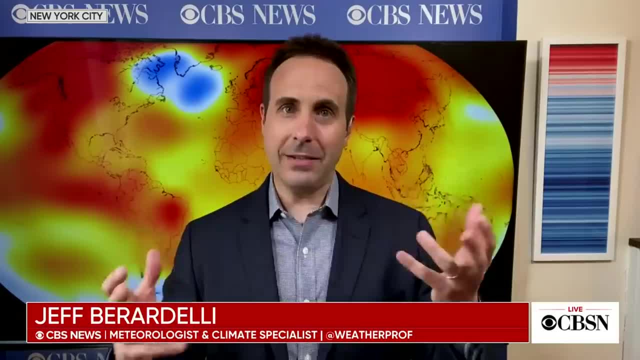 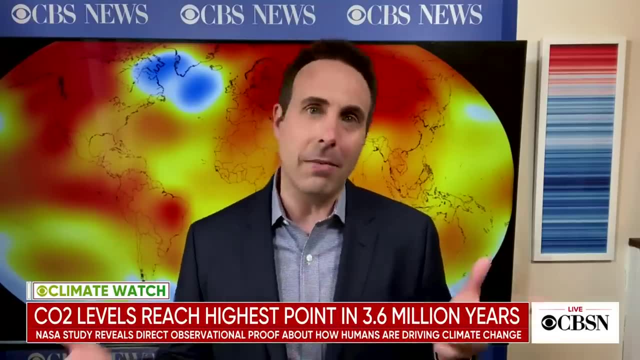 even if we put less money in this year, it doesn't mean that we see less money in the bank overall. It's like a savings account: It keeps accumulating, Unfortunately. so even though our emissions went down by 5 to 7 percent, it's kind of negligible because we're 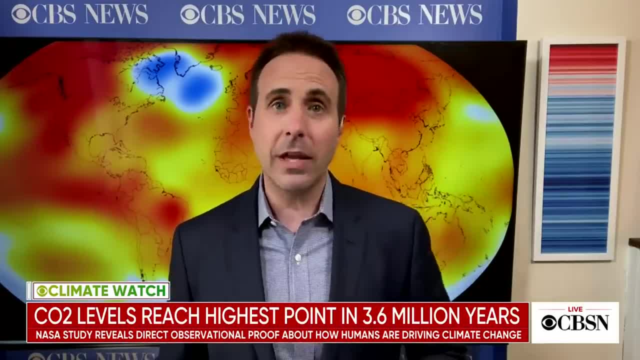 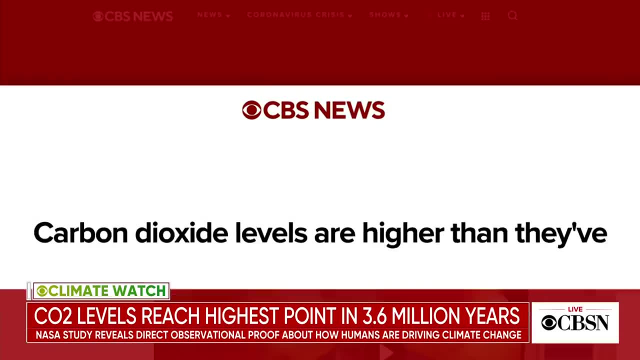 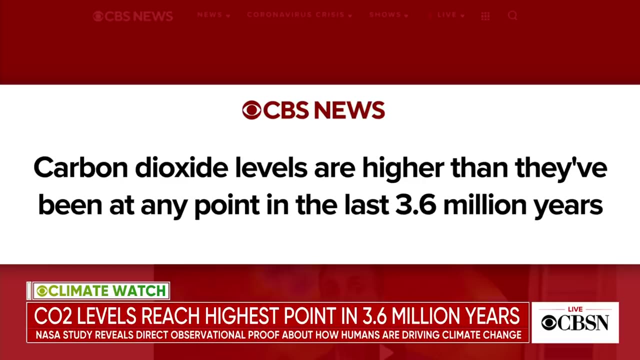 still adding more emissions into the atmosphere, And so the level has hit another record high, the highest it has been in 3.6 million years. And, by the way, Lana, it is increasing at 100 times the pace that it naturally should Think about that and how we've transformed the Earth. 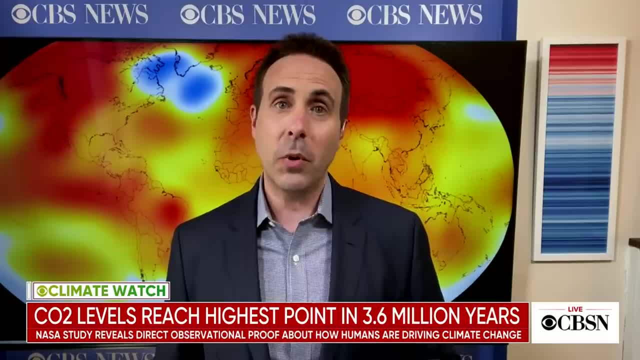 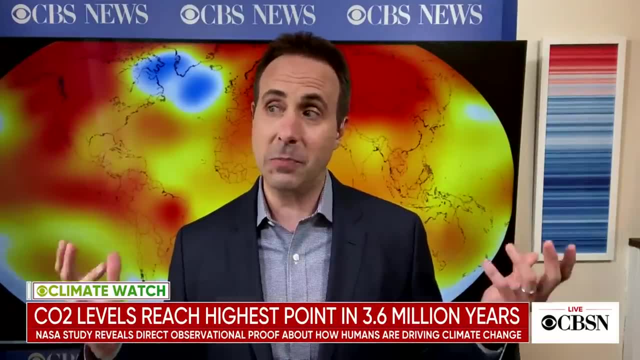 in just a short 150, 200 years, We've put 50 percent more carbon dioxide into the atmosphere, into the atmosphere. And so I like to say we're kind of like guinea pigs on an experiment that we do not know what the end result will be, But we have a good idea that that end result is not good. 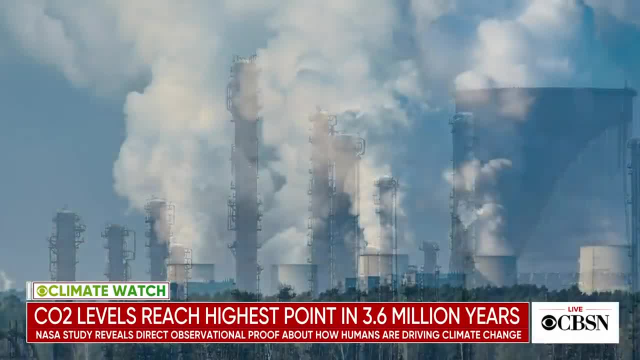 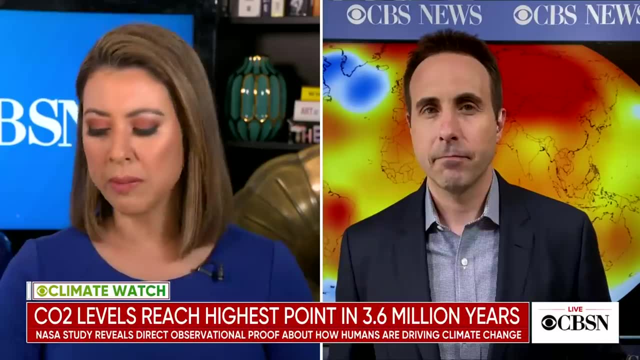 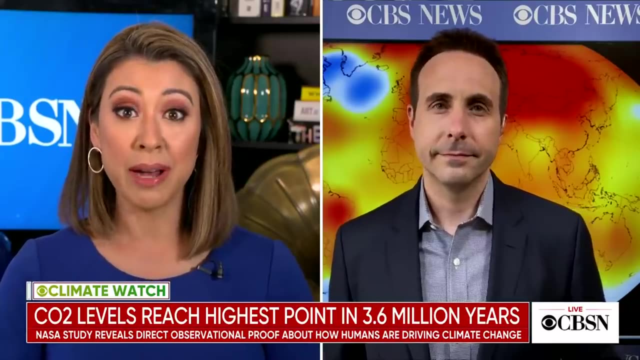 unless we start curbing our emissions. Well, Jeff, I want to get back to the study in just a minute, But but to stay with you on this for a second. we're seeing more automakers pledge to electric cars. We are seeing other corporations make green pledges, But when we've when. 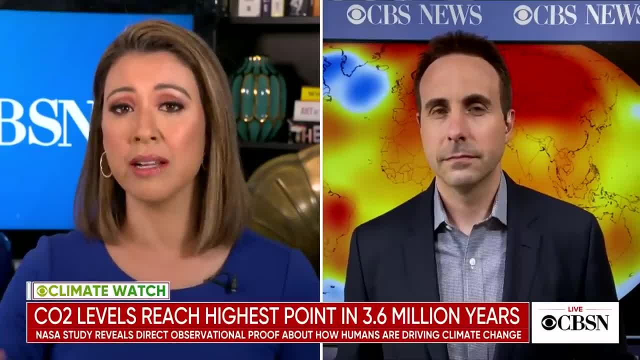 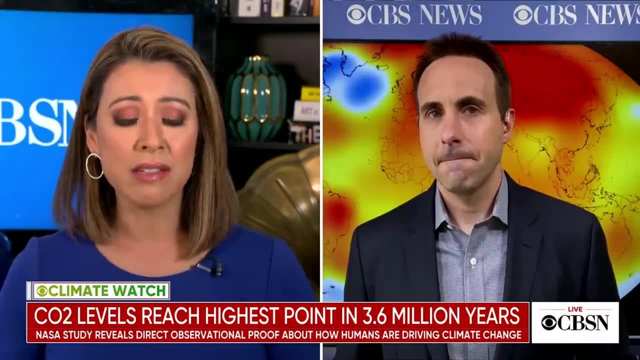 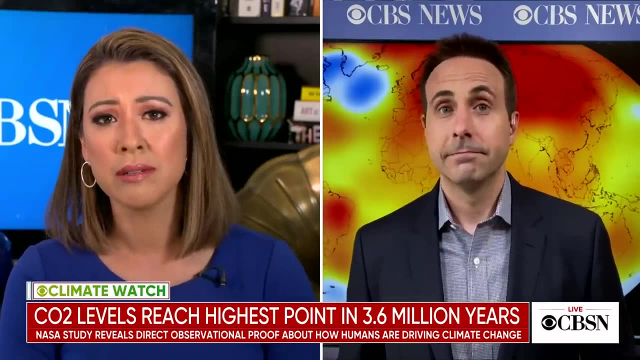 you say, as you do, that it's it's cumulative and the pace is is is accumulating so fast. What hope does does all of these measures actually give us for being able to to pump the brakes a little bit on climate change? I like the pun: pump the brakes. That was good, So you know. 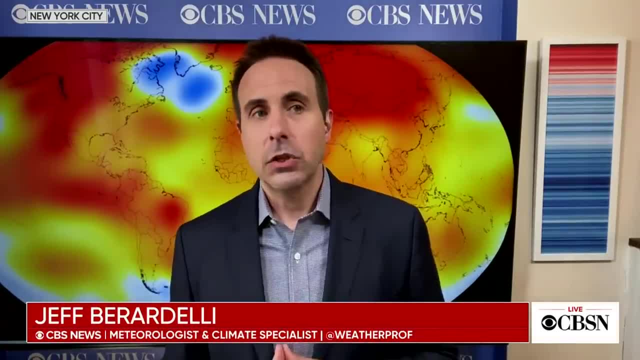 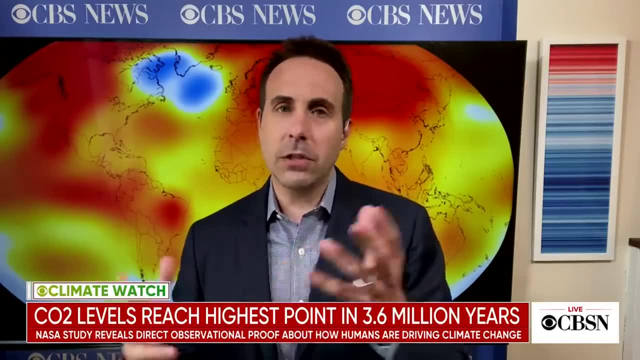 basically, anything helps, We have to do something right. So transportation accounts for about 25 percent of the population, And so we're seeing more automakers pledge to electric cars, And so the greenhouse gas emissions in the United States we have to pair. Let's say we took all the EVs. 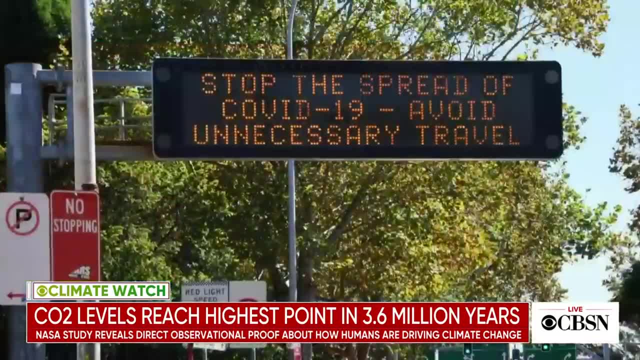 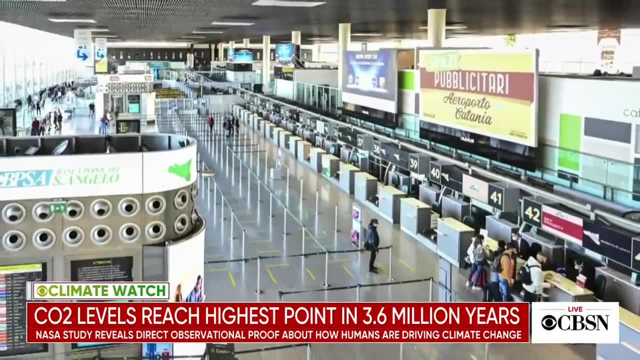 We took all the gas powered cars off the road and it was just EVs. So cars and trucks that were, that were powered by electric. We'd have to pair that with the electric grid being completely renewable. So 25 percent in transportation, around 30 percent in electricity. So the power. 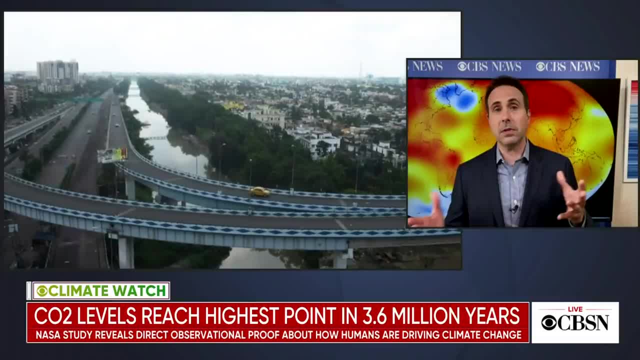 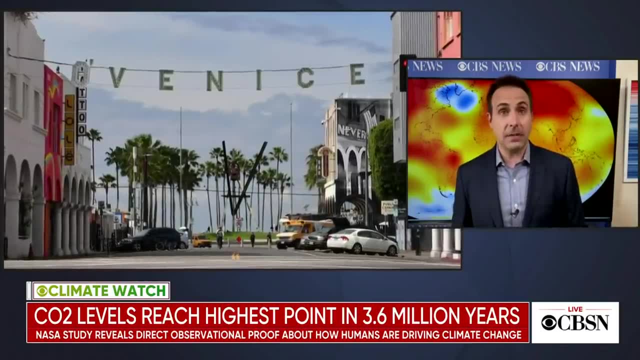 production is around 55 percent, So we'd be able to reduce emissions by about 50 percent. That's just here in the United States, But let's say everybody in the world does it. We'd see a decrease in emissions by 50 percent or so. Now remember, stuff is still. 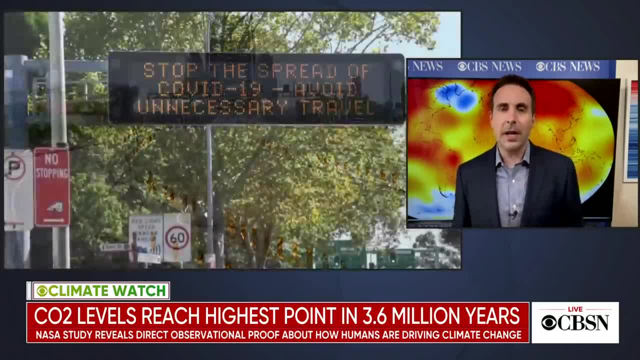 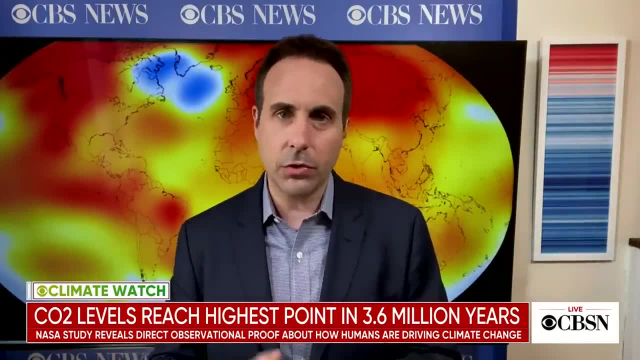 accumulating in the atmosphere And like a bank account it goes up and up, But we would at least have reduced the amount of emissions. And then we have to continue to do other stuff in agriculture and in the production of cement and steel and airplanes and all that stuff to bring it down. 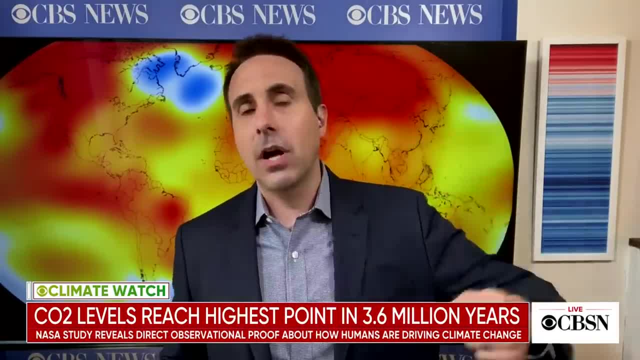 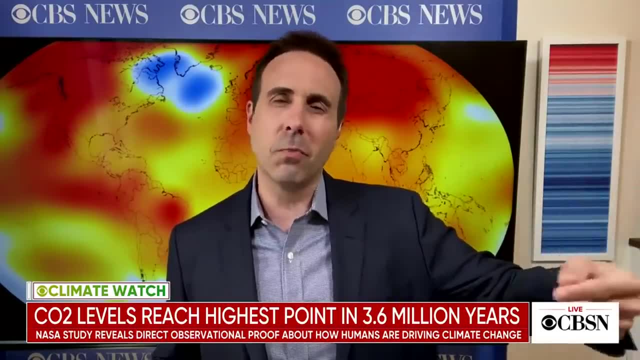 even further over the course of time And at that time we will also be ramping up what's called carbon capture so that you know, sometime around the year we're going to be able to do that. So let's say, you know, in the 2030s, more so the 2040s, 2050, we could start pulling carbon dioxide. 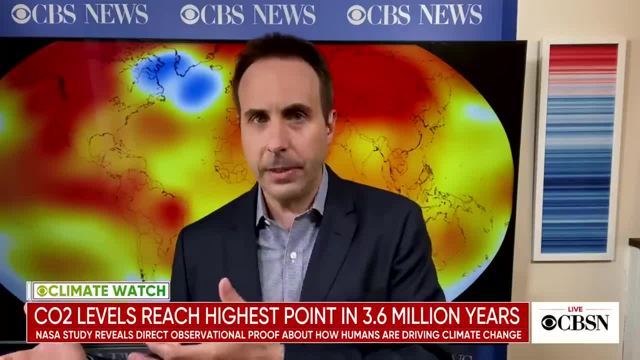 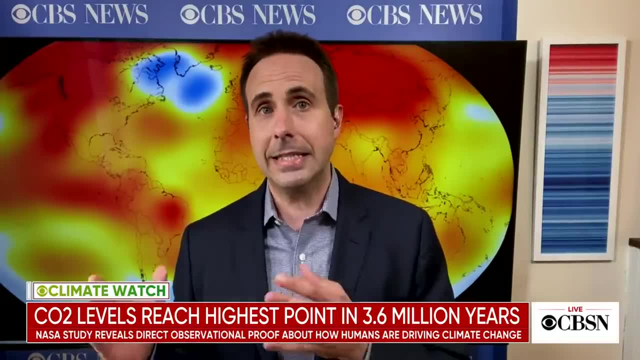 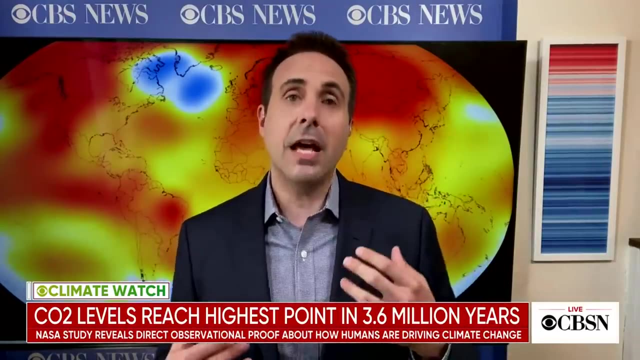 back out of the atmosphere to try to reduce eventually the temperature of the earth, because we've increased temperatures by around about two degrees Fahrenheit since the early 1900s, late 1800s or so. So we just have to do our best right now to reduce emissions and then do our 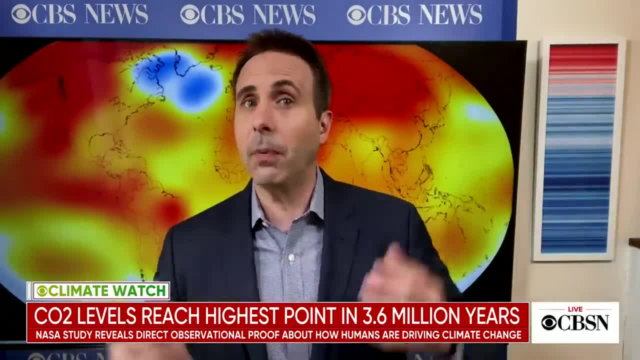 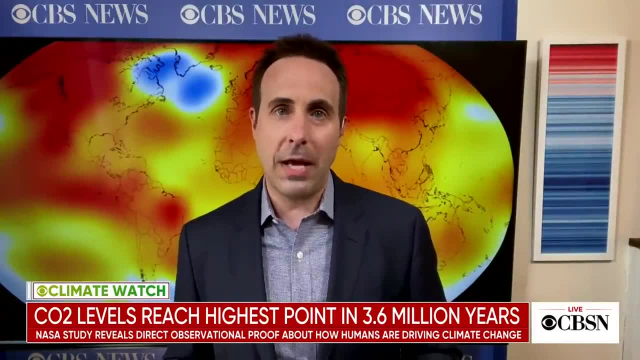 best right. you know, in a couple of decades or so, once the technology is up to par, to start pulling carbon dioxide and methane back out of the atmosphere. So it's a gradual process, but we have to do everything we can right now to limit warming as fast as we can and getting cars off. 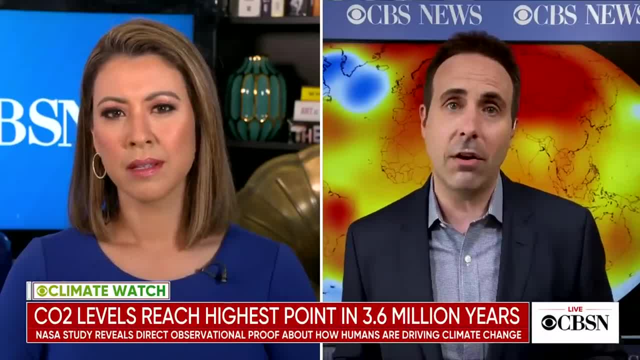 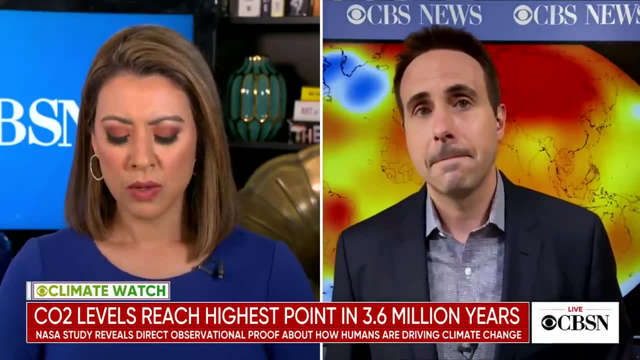 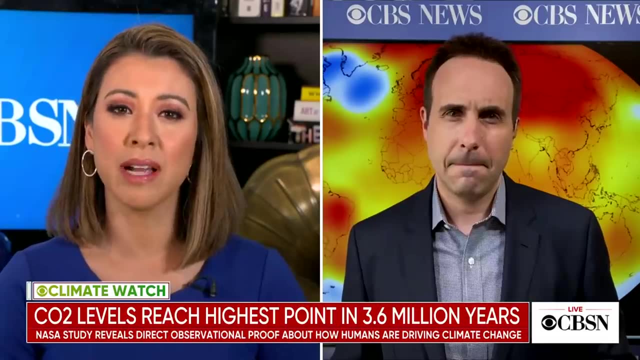 the road and also using renewable energy in our energy system is going to do. it's going to be a huge accomplishment if we can accomplish that. Well, Jeff, let's go a little bit deeper into this particular study. Tell us what makes it the first of its kind and what piece of the climate. 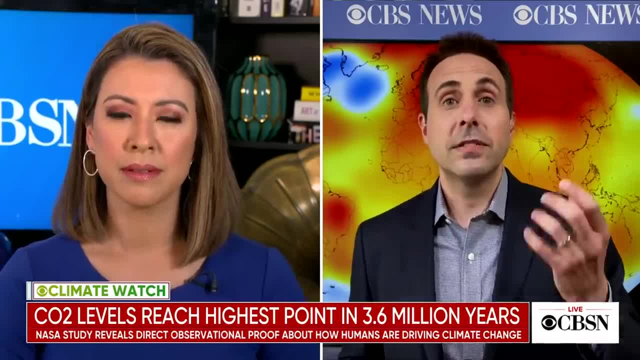 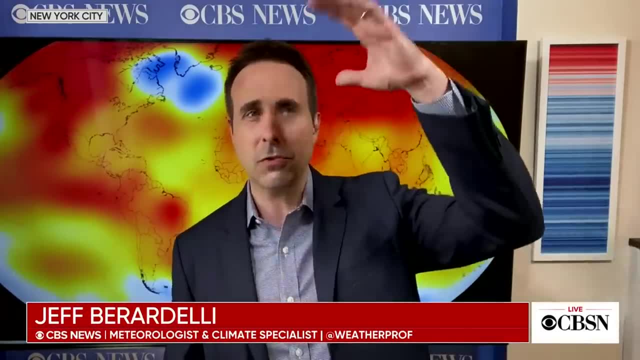 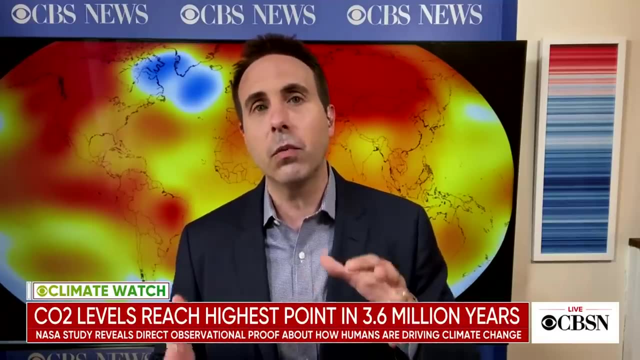 change puzzle it fills. So this NASA study is really interesting, right? So we've known for decades and decades tons of scientific research- you can pile it up to probably the moon- that says that carbon dioxide and methane are warming the atmosphere, but we've never been able to measure it directly. 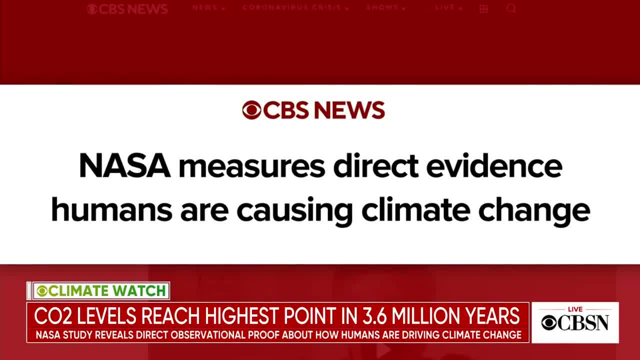 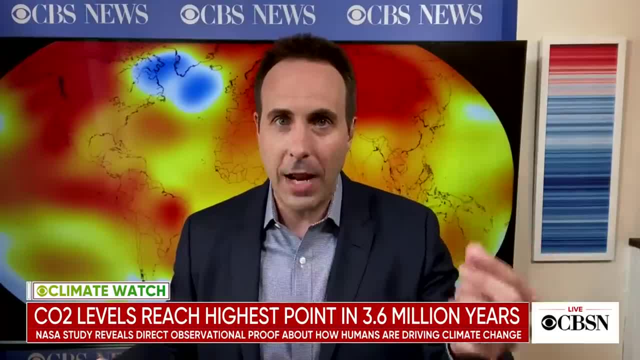 We've been able to measure it in labs, but we haven't been able to measure it in the real world, on the earth, at least as a whole. Well, NASA has been able to do it now, finally getting direct observations, quantifying the impact of increased greenhouse gases by using satellite measurements. 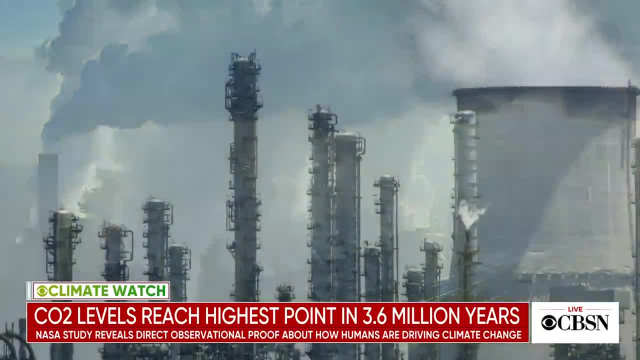 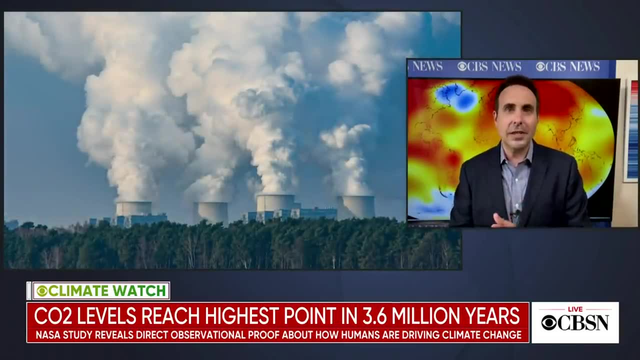 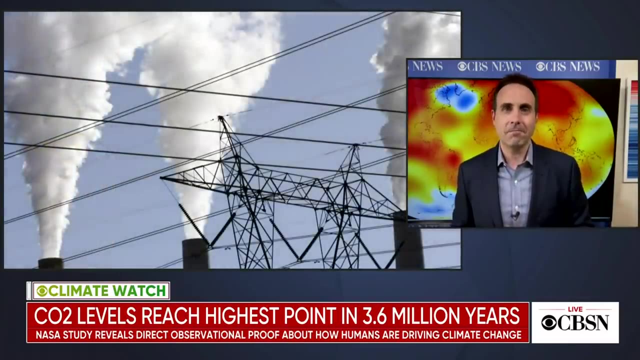 So they now have the proof that climate change is caused by humans. We were 99.99% sure, but this certainly tells us for certain that humans are causing climate change and there's really no way around it. It's the gold standard of scientific credibility in research. 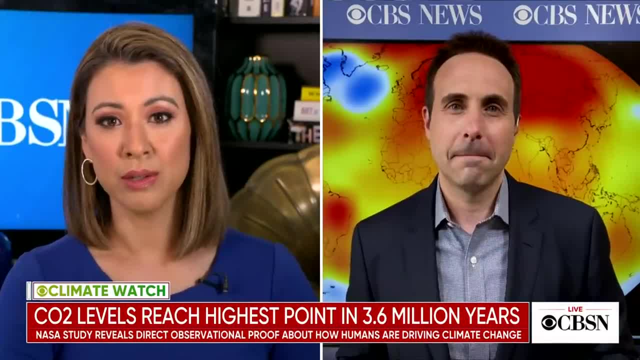 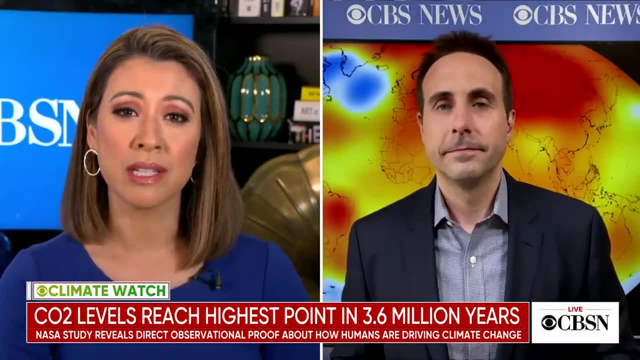 Well, you are someone who has been watching this science closely for some time. Do you think that climate change is gaining relevance when it comes to corporations addressing social issues? We're seeing in this case, NASA and the government say definitively: this is what's. 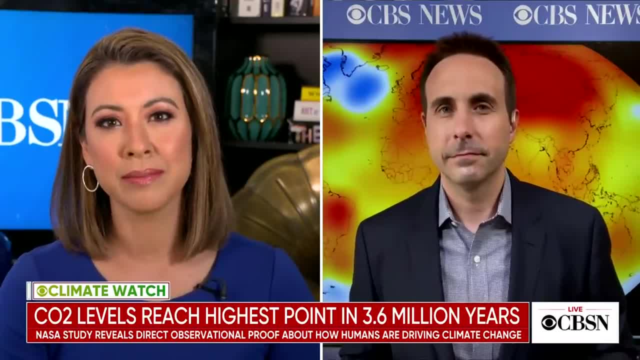 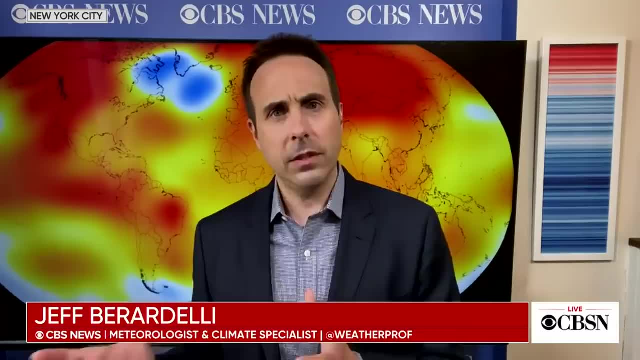 happening, How is the rest of society responding? Well, it's really amazing what has happened over the past few years. It really is incredible. Just a couple of weeks ago, maybe about a week ago or so, 300 corporations signed a pledge to stop climate change And they signed a pledge to stop climate. 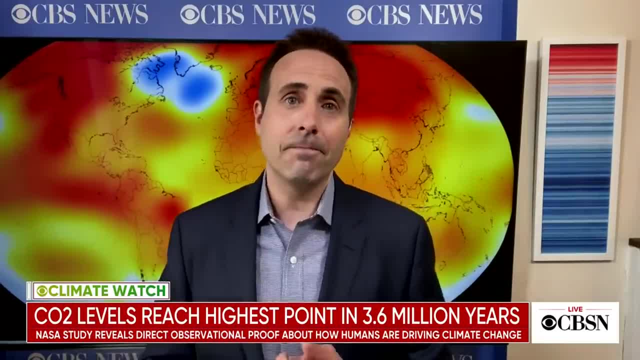 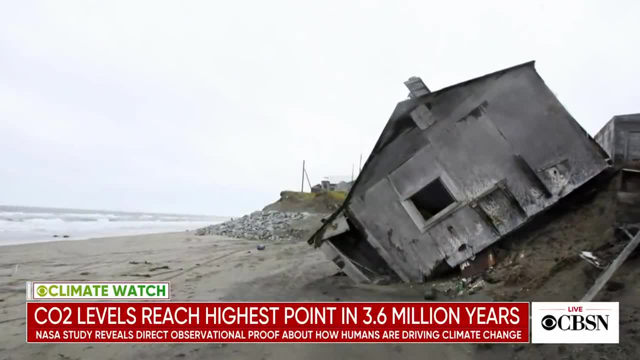 change And they signed a pledge to stop climate change. And they signed a pledge asking the Biden administration to double their what we're offering as far as the amount of emissions that we're going to cut to the Paris Agreement. So they are asking for more bold action from the Biden. 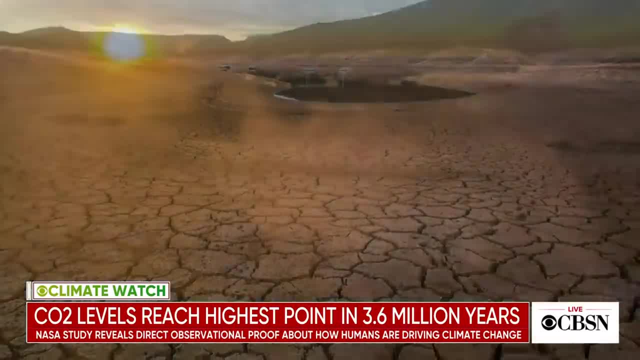 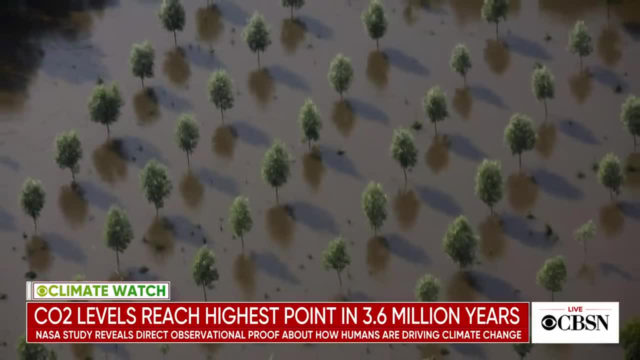 administration. That wasn't necessarily the case just a few years ago. So we definitely are seeing corporations step up, And I think a lot of that is due to pressure from consumers. Consumers are becoming aware They want their corporations to be more responsible, And so corporations are.